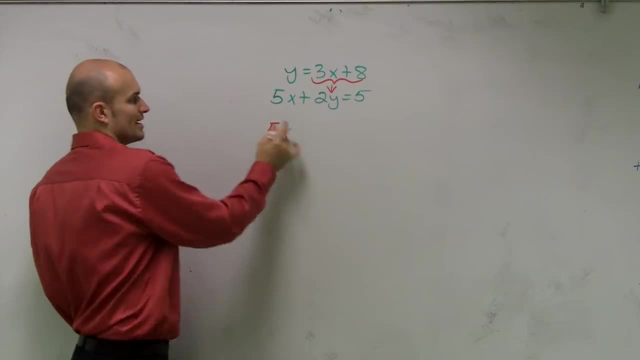 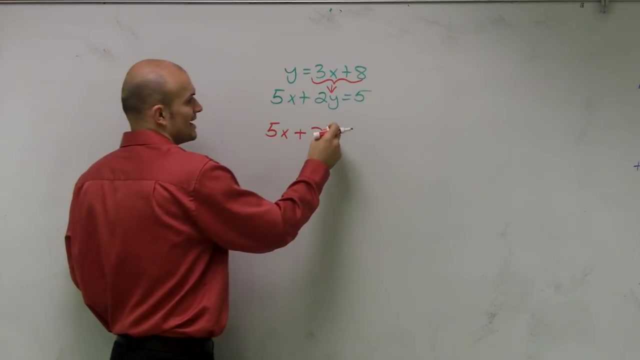 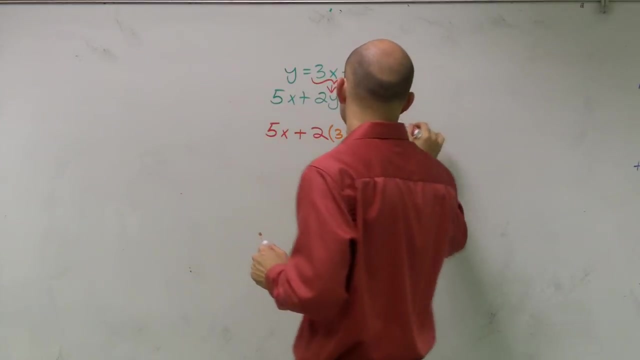 in for my variable in the other equation. So I can say 5x plus 2, and instead of writing 2 times y, which would be that second equation, I can write it times 3x plus 8. plus 8 equals 5.. 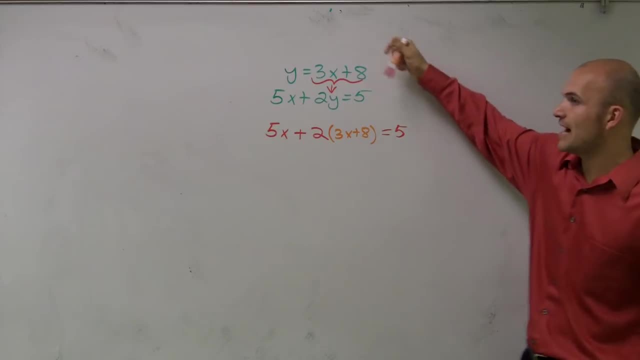 So does everybody see what I did? All I simply did is I took the value of my variable- it doesn't matter which variable- and I took that value of it and I substituted it in for the variable in the other equation. Okay, 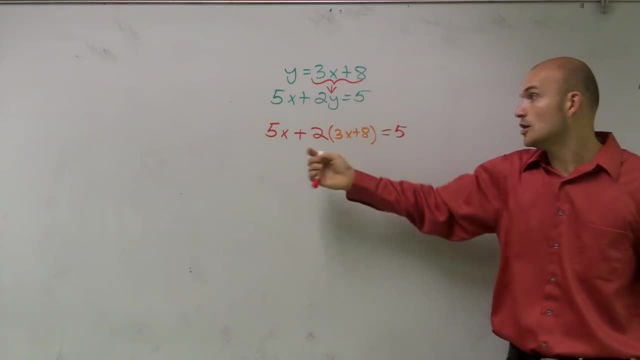 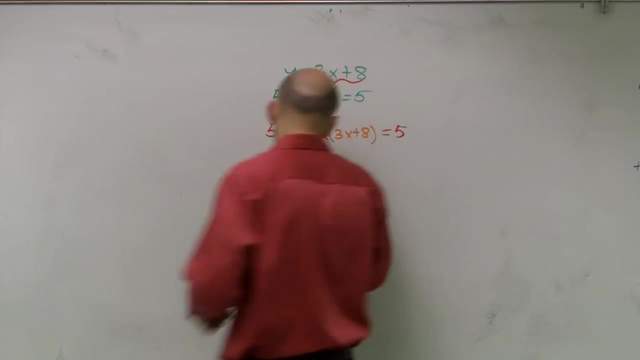 So then, once I have that, you can see. now I have an equation with the same variable. So now it's going to be something I can solve for. So remember, when we have a number of multiple parentheses, we need to use distributive property. 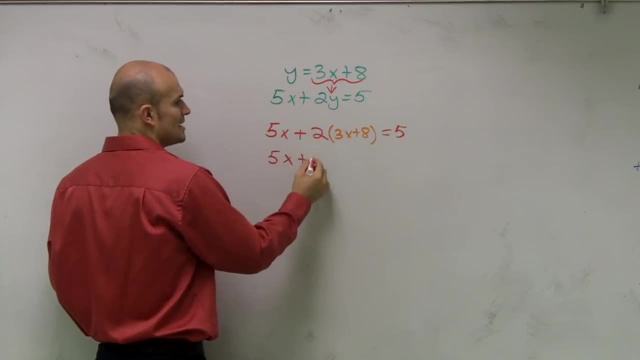 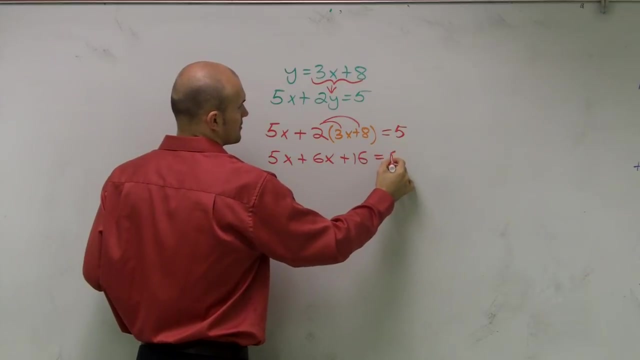 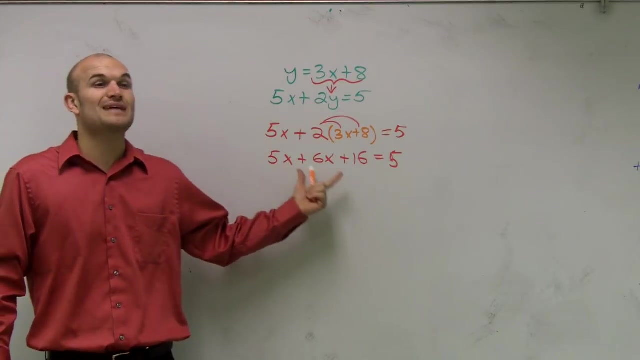 So therefore, I have 5x plus 2 times 3x is 6x. 2 times 3x is 6x. 2 times 8 is a positive 16 equals 5, all right. The next step I want to do, guys, is remember when you have your variable. 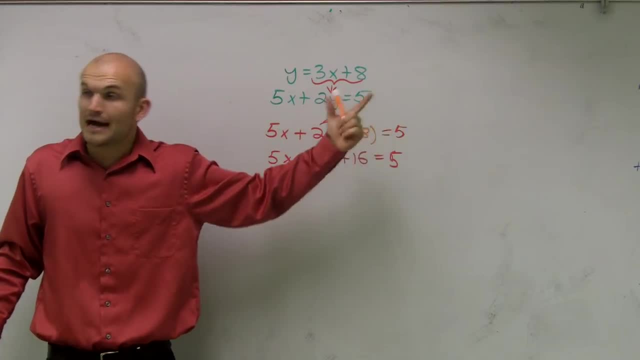 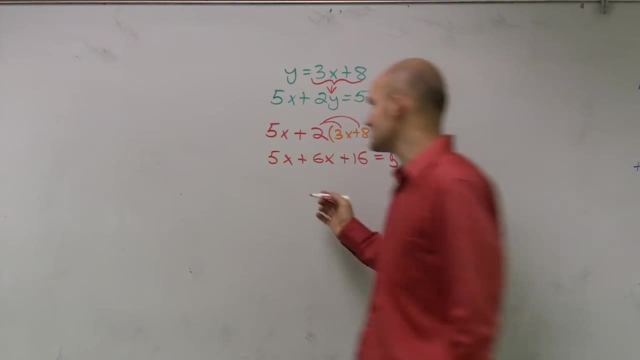 on the same side of your equation, not on opposite sides. On opposite sides you need to do the add and the subtracting, But when they're on the same side you just combine like terms: 5x plus 6x is 11x plus 16 equals 5.. 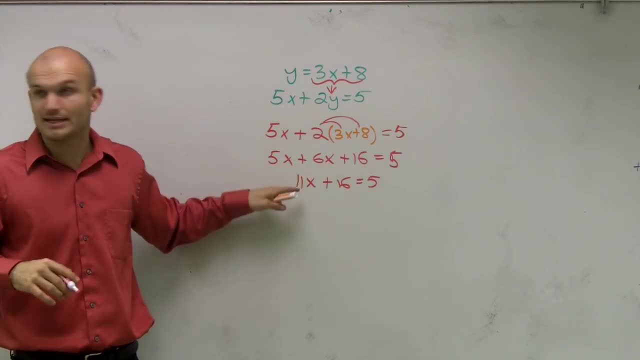 Now it's a two-step equation. I need to get my rid of my 6x, I need to get rid of my 16 and get rid of my 11.. The 16 is added to my variable, so I subtract 16 on both sides. 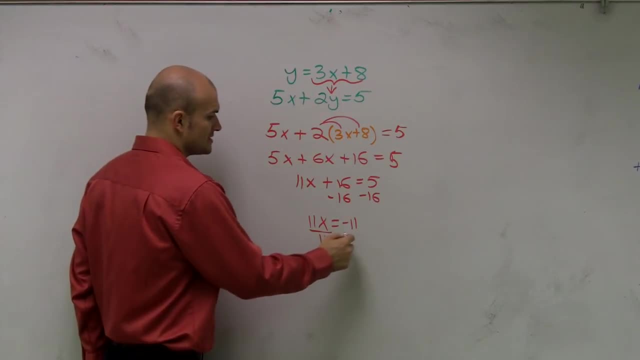 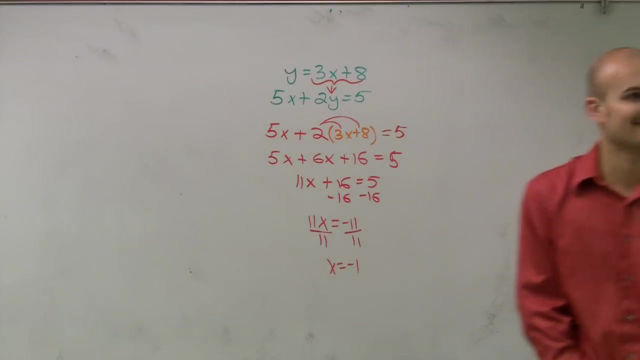 Now I have 11x equals negative 11, divide by 11, on both sides, x equals a negative 1, right, Okay, So since my x now equals negative 1,. remember, guys, when we were talking about the graphing. 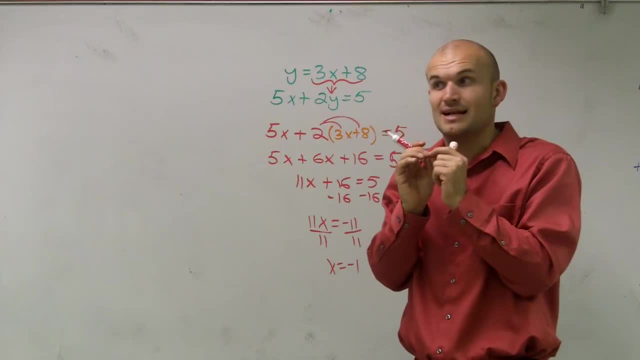 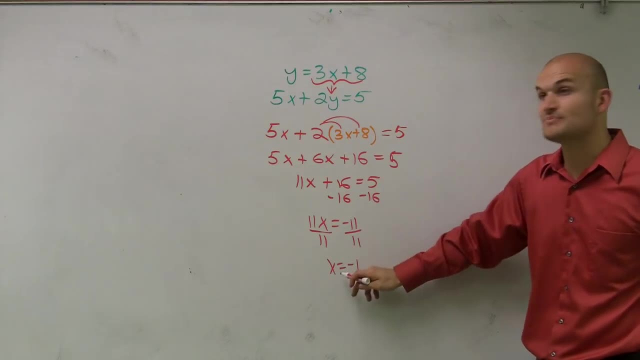 remember there was an x and a y coordinate right. Their intersection point intersected at a given point: x comma y. So if I know what the value of my x, now what I need to do is substitute that value back into one of my equations. 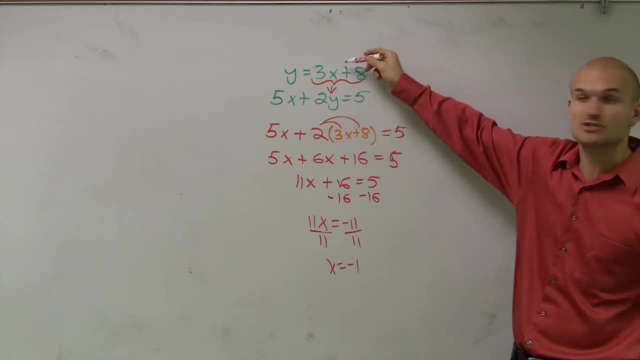 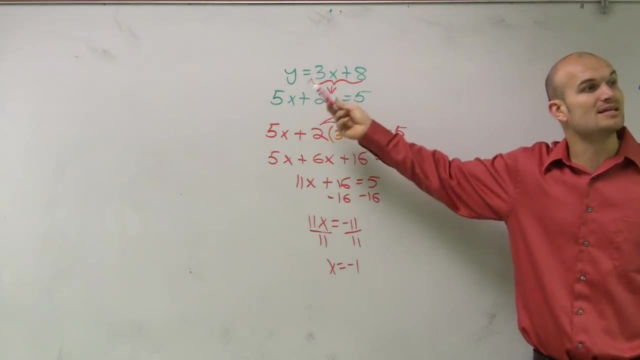 Now a lot of students want to substitute it into the second equation, because that's what you substituted your first variable for. right, It makes sense: Plug negative 1 in for this x. But what I'm telling you is: it doesn't matter which equation you substitute your value in for.